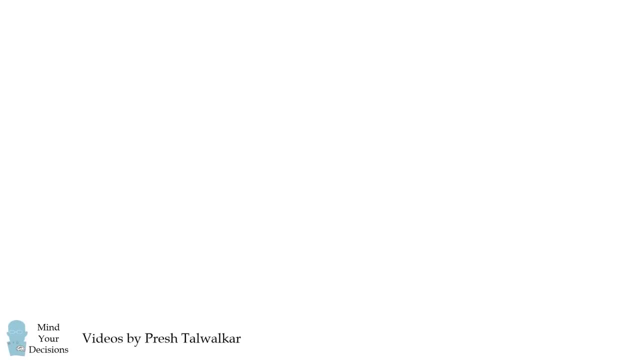 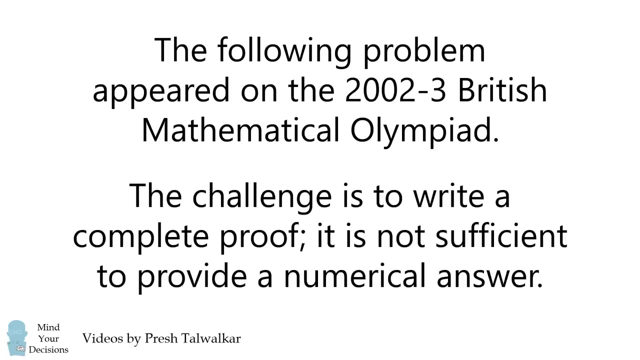 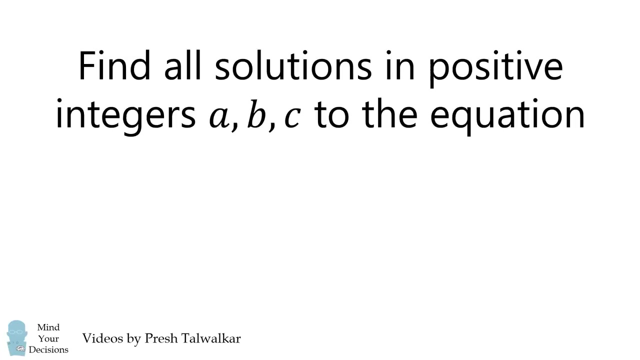 Mind your decisions. I'm Presh Talwalkar. The following problem appeared on the 2002-2003 British Mathematical Olympiad. The challenge is to write a complete proof. It is not sufficient to provide a numerical answer alone. Bind all solutions and positive integers a, b and c to the equation. 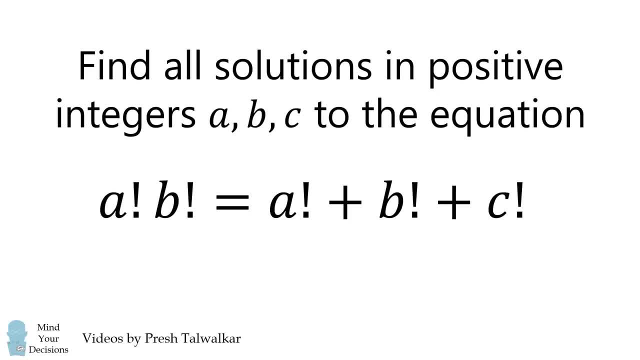 a factorial multiplied by b factorial is equal to a factorial plus b factorial plus c factorial. I thank Nahian for the suggestion. Pause the video if you'd like to give this problem a try and, when you're ready, keep watching to learn how to solve this problem. 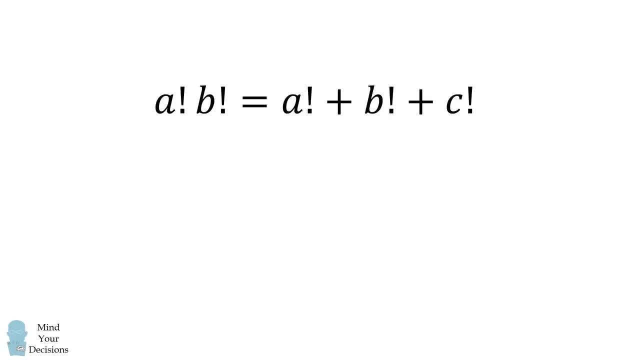 We will get started by noticing a symmetry in this equation. What would happen if we transpose the variables a and b? Because multiplication and addition are commutative, we have an equivalent equation. Therefore, if a, b, c is a solution, then we know b a c is also a solution. 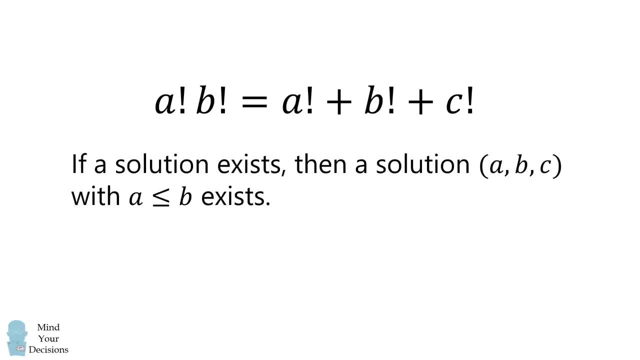 What this means is that if a solution exists, then a solution- a, b, c- with a less than or equal to b- also exists. Without any loss of generality, we can suppose a is less than or equal to b. The proof will proceed in the following form: 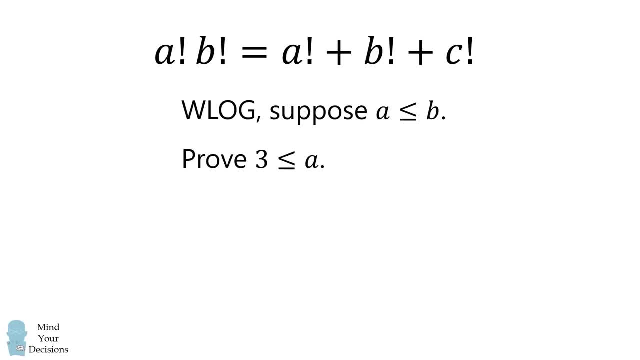 First we'll prove that 3 is less than or equal to a, then we'll show that b is less than c, then we'll prove a is equal to b and finally we'll prove c is less than or equal to a plus 2 and solve for the numerical answer. 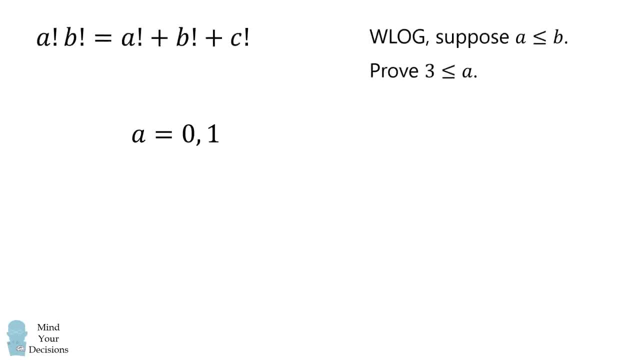 Let's get started by working out a few cases. Suppose a is either 0 or 1, then a factorial is equal to 1.. We substitute that into the original equation and then simplify. This equation only has a solution if 0 is equal to 1 plus c factorial. 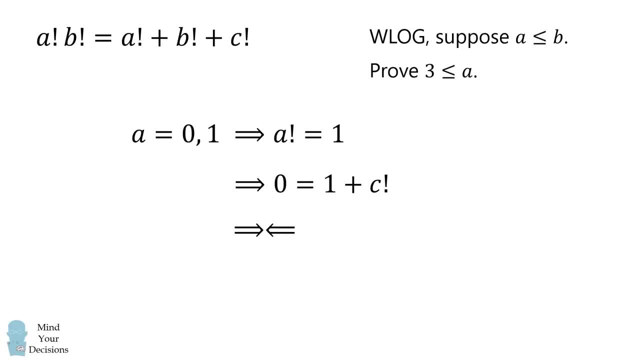 But no solution exists for this equation where c is a positive integer. Therefore a cannot be equal to 0 or 1.. We then consider the case a is equal to 2. This means a factorial is also equal to 2.. We substitute that in and then we simplify the equation. 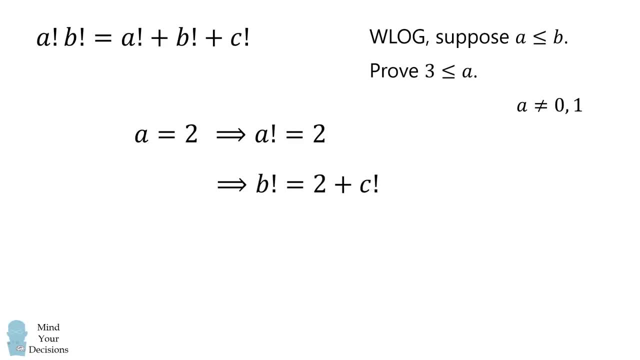 Notice, there is no factorial that's 2 more than another factorial, because the factorial sequence goes in order: 1,, 2,, 6, and so on. Therefore, this equation also has no solutions for integers b and c. Therefore a cannot be equal to 2.. 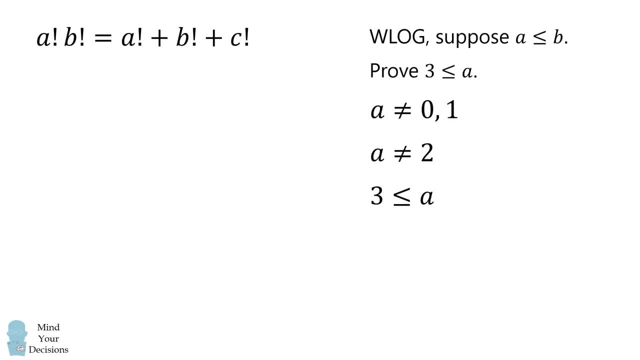 This means a has to at least be equal to 3.. Then we suppose that a is less than or equal to b, so we can add that onto the inequality. From here we are going to prove that b is less than c. To do that, we'll assume the opposite: b is greater than or equal to c, and then 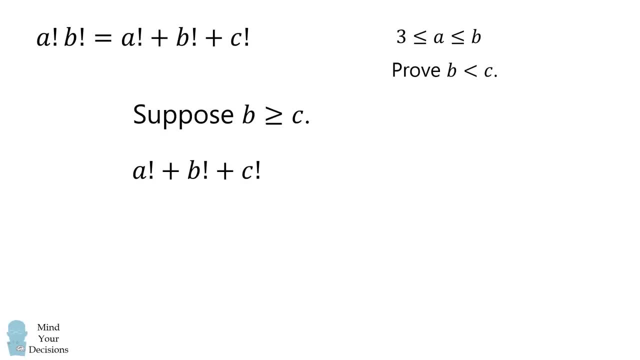 derive a contradiction. We can bound the sum a factorial plus b factorial plus c factorial as follows: We have assumed that a is less than or equal to b, therefore a factorial will be less than or equal to b factorial, Then b factorial is equal to b factorial. 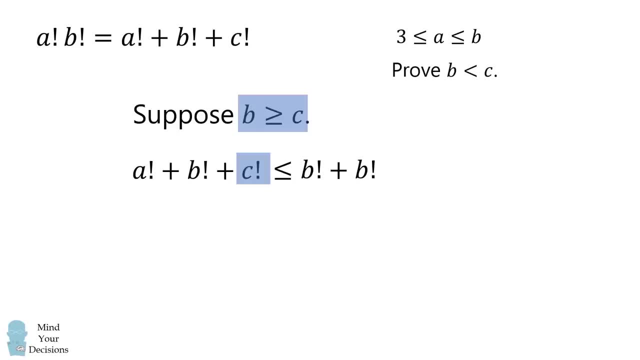 We can then bound c factorial because we have supposed that c is less than or equal to b. therefore c factorial will be less than or equal to b factorial. This sum will be equal to 3 multiplied by b factorial. so we have an upper bound on. 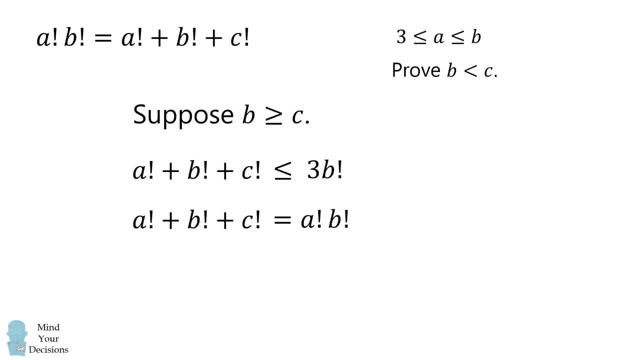 the sum, But we can also derive a lower bound. This sum is equal to a factorial multiplied by b factorial. We know that a is at least equal to 3, which means this is at least equal to 3 factorial multiplied by b factorial, which is equal to 6 multiplied by b factorial. 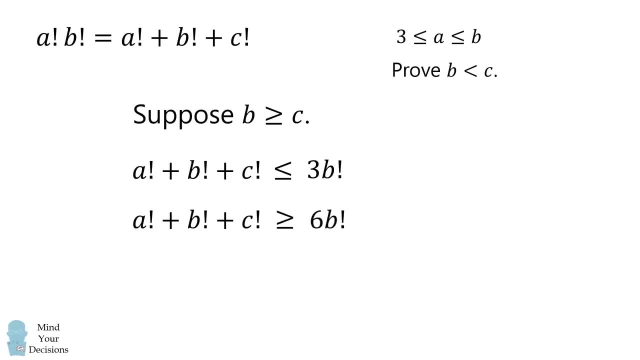 Therefore, we've shown the upper bound of the sum is actually lower than the lower bound, and that's a contradiction. Therefore, our assumption that b was greater than or equal to c must have been wrong, and we've shown that b is less than c. 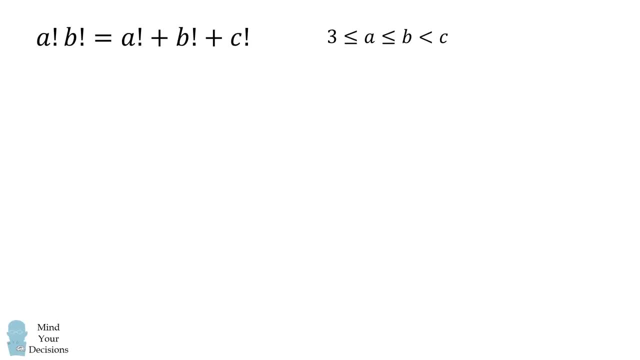 Before we proceed to the next part of the proof, I'm going to go over a bit of notation. This notation means that m divides n. It's equivalent to saying n is divisible by m. It's equivalent to saying n is a multiple of m. 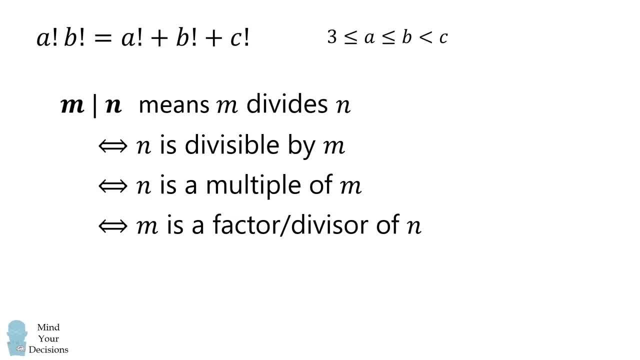 And it's equivalent to saying that m is a factor or divisor of n, 2 divides 4,, 3 divides 12, but 2 does not divide 5.. Now let's show that a is equal to b. To do that, we'll assume the opposite, that a is not equal to b. 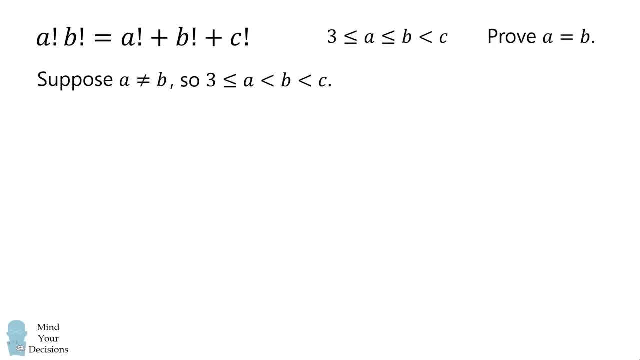 This means 3 is less than or equal to a which is less than b which is less than c. So we go to our original equation and we'll divide both sides by a factorial. This simplifies to be the following equation: 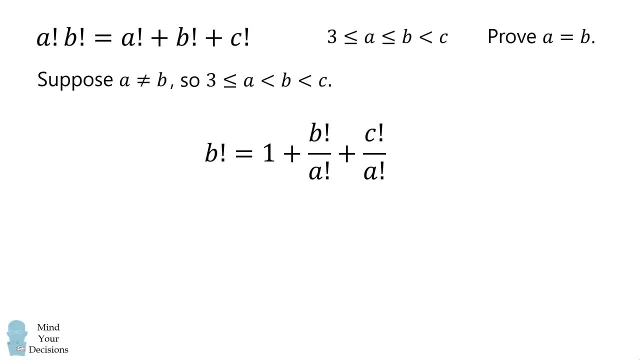 Notice, the left hand side is b- factorial and the right hand side will be the sum of three integers. This is because b and c are greater than a, So b- factorial over a factorial is an integer and c- factorial over a factorial is an integer. 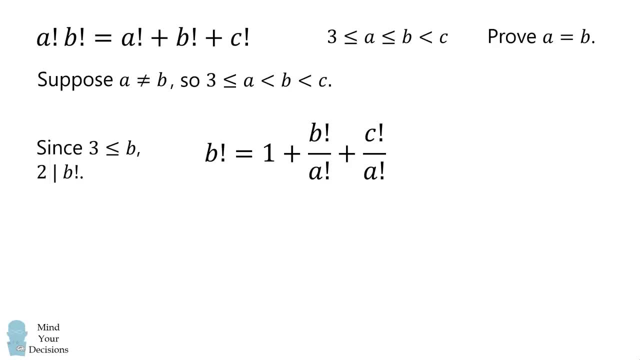 Now, since b is at least equal to 3, we know that b factorial is less than or equal to 3.. And b factorial is an even number. That's because every factorial above 3 factorial will be an even number. Consequently, the entire right hand side, which is the sum of integers, has to be an. 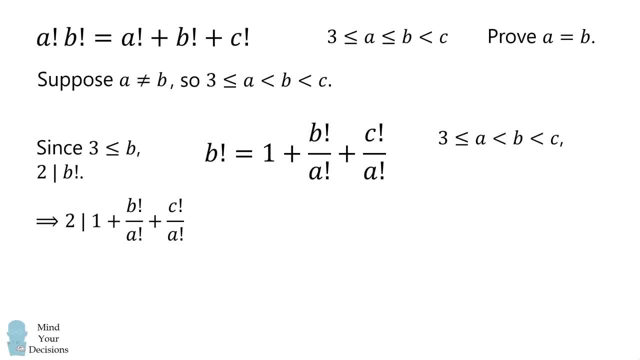 even number. Now, since 3 is less than or equal to, a is less than, b is less than c, we know that b is at least equal to a plus 1, and c is therefore at least equal to a plus 2.. 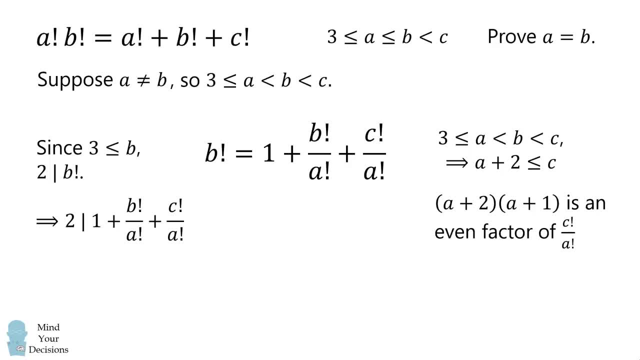 But then a plus 2 multiplied by a plus 2 is equal to a plus 2.. So b factorial over a factorial is an even number, But then a plus 2 multiplied by a plus 1 must be an even factor of c factorial over. 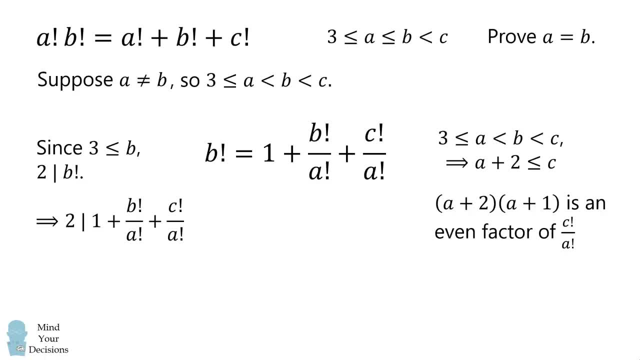 a factorial. That's because the product of any two consecutive numbers is an even number. Consequently, 2 divides c factorial over a factorial. Now, in order that the entire right hand side be an even number, we must have 1 plus b factorial. 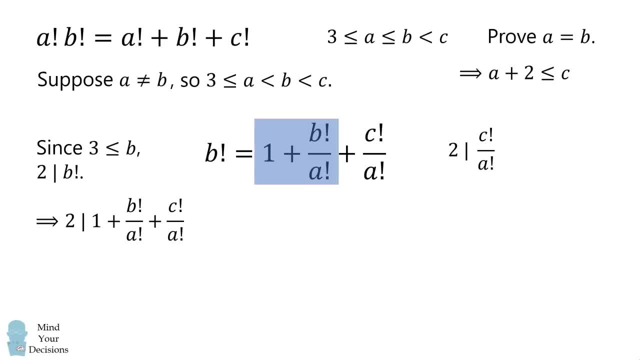 over a factorial is an even number, But 1 is an odd number, which means we must have an odd number plus an odd number. So b factorial over a factorial must be an even. number over a factorial must be an odd number. Now, since b is greater than a, this implies that b is equal to a plus 1.. 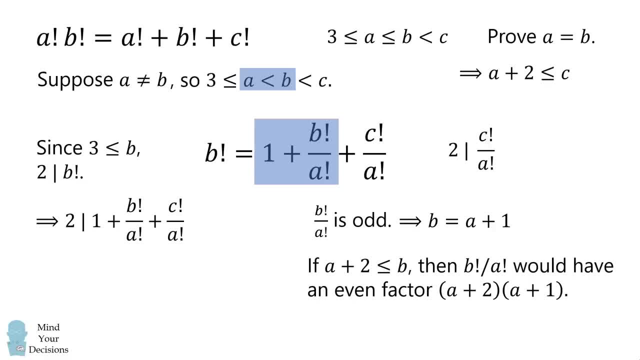 The reason is that if b was at least equal to a plus 2, then it would have an even factor of a plus 2 multiplied by a plus 1, which is not possible since b- factorial over a factorial, is an odd number. So from here let's consider what happens if b is equal to a plus 1.. 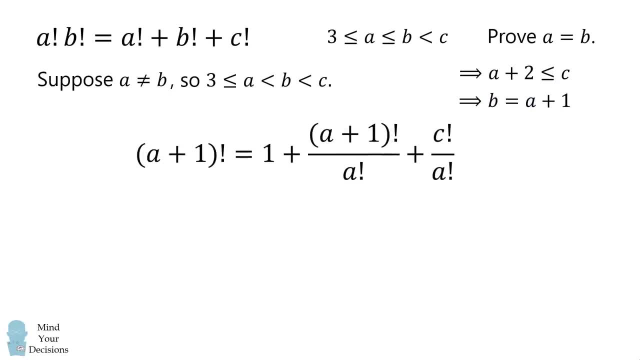 We'll substitute that into our equation and we'll simplify. We now consider the divisibility of this equation by the factor a plus 1.. The left-hand side is a plus 1 factorial. Naturally it has a factor of a plus 1.. 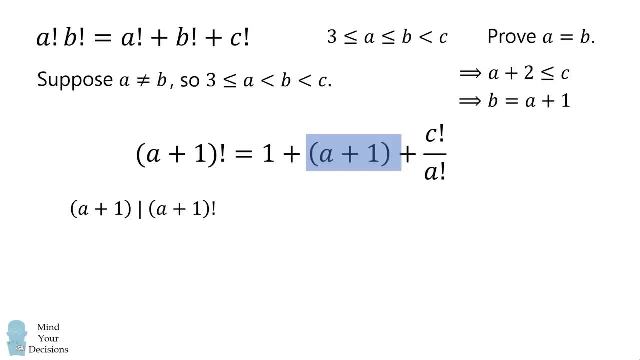 The right-hand side will be the sum of three integers. Naturally, a plus 1 has a factor of a plus 1.. Now c, factorial over a factorial, will also have a factor of a plus 1, because c is at least equal to a plus 2.. 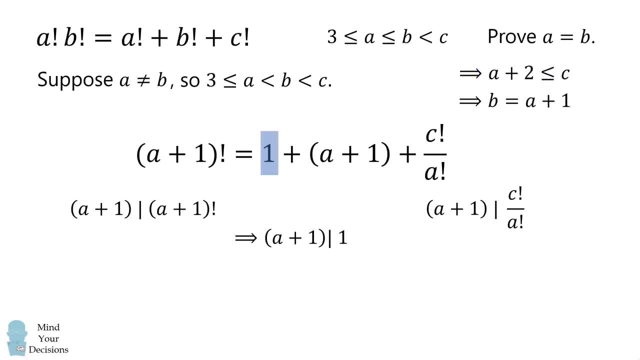 Therefore, for the right-hand side to be divisible by a plus 1,, we must have a plus 1 divide 1.. But that means that a is equal to 0, and that's a contradiction, because we know that a is at least equal to 3.. 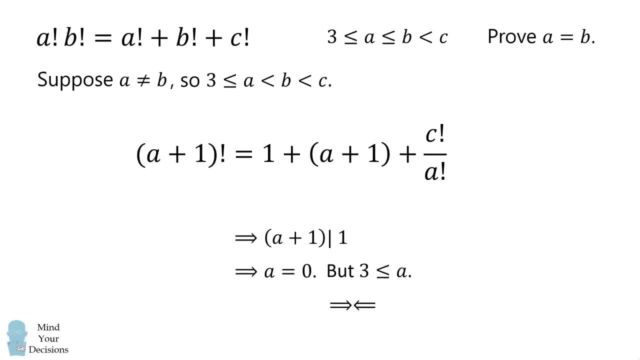 Therefore, our original assumption was wrong. We cannot have a is not equal to b. We must have a is equal to b. We will then consider the next step Over here we want to prove that c is less than or equal to a plus 2.. 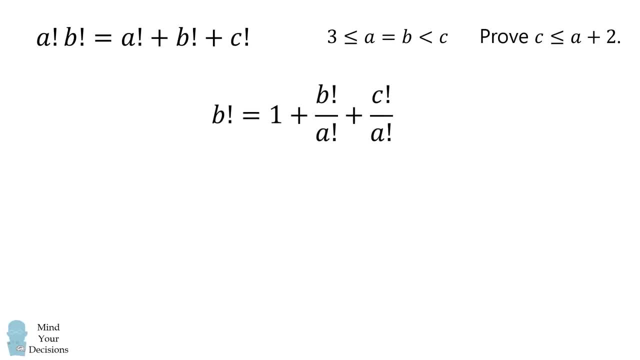 We'll again take our original equation, divide both sides by a factorial. We're going to substitute that a is equal to b and then we'll simplify this equation. We'll simplify it a little more and then we'll subtract 2 from both sides. 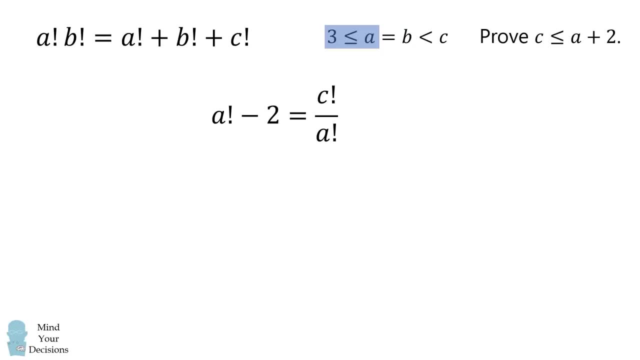 We'll again look at divisibility. Since 3 is less than or equal to a, we know that a factorial is divisible by 3.. However, we then know that a factorial minus 2 is not divisible by 3.. This is because a factorial is a multiple of 3, and we're subtracting 2 from it. 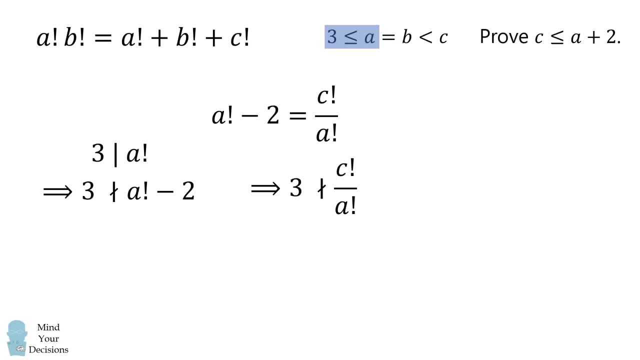 Therefore 3 does not divide a factorial minus 2, which means 3 cannot divide c factorial over a factorial. Now if c was greater than or equal to a plus 3, then c factorial over a factorial would have a factor of a plus 3 multiplied by a factorial. 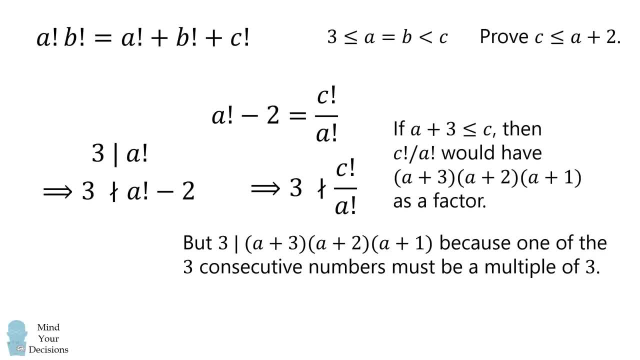 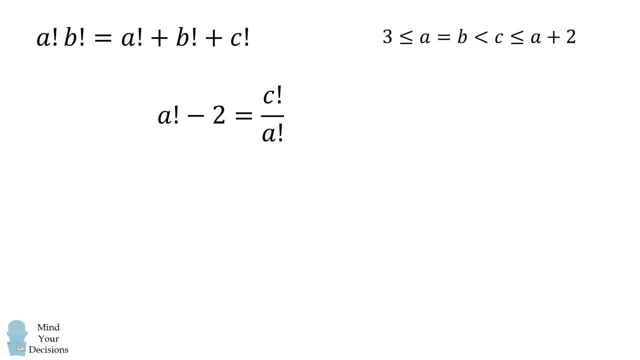 But 3 would divide this product, because one of three consecutive numbers must be a multiple of 3.. Therefore, we must instead have c being less than or equal to a plus 2.. So we only have two possibilities to consider: Either c is equal to a plus 2, or c is equal to a plus 1.. Let's consider each one in turn. 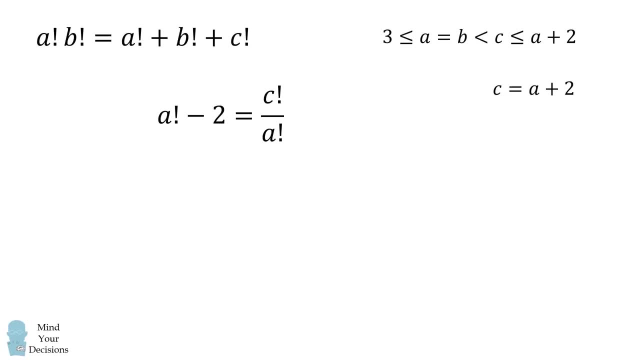 Suppose c was equal to a plus 2. We'll substitute that into the equation. We'll then simplify this, and now we'll do a little bit of algebra. We'll multiply on the right-hand side and then we'll take all of the a terms to the left and put all the constant terms on the right. 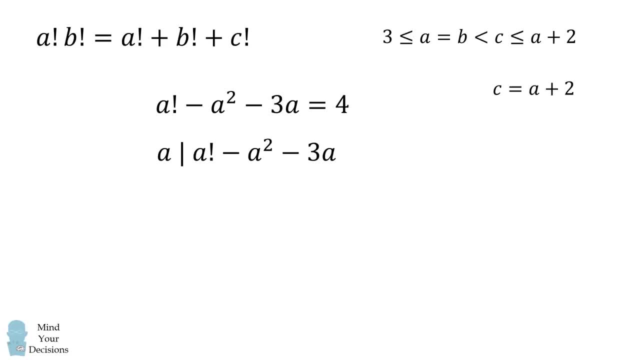 Now in this equation, notice that every single term on the left-hand side of the equation is divisible by a. This means that 4 has to be divisible by a, But since a is greater than or equal to 3, the only way this is possible. 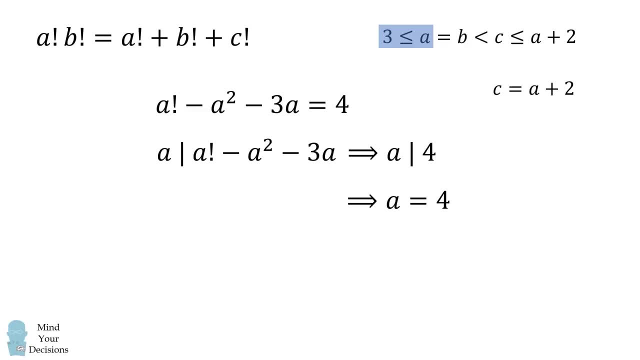 is if a is equal to 4.. So let's substitute: a is equal to 4, b is equal to a, which is equal to 4, and then c is equal to a plus 2. So c is equal to 6.. 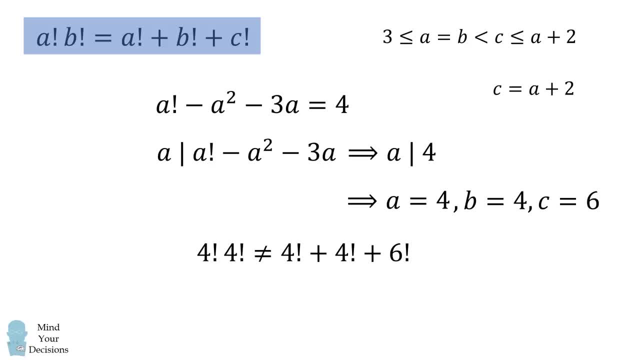 Well, if we substitute that into the original equation, we actually get something that does not work. 4 factorial multiplied by 4 factorial is not equal to 4 factorial plus 4 factorial plus 6 factorial. Therefore c is equal to a plus 2. It does not lead to a solution. 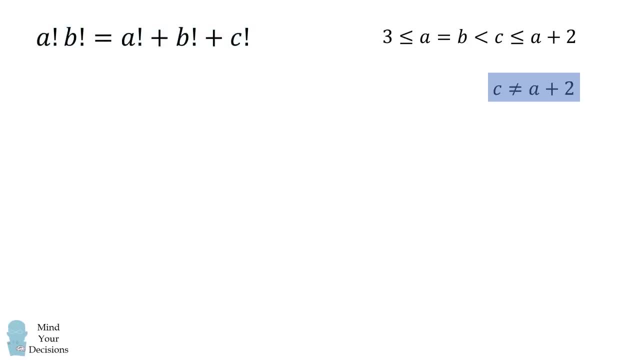 So we instead need to consider the other case, that c is equal to a plus 1. Now, in this case we'll substitute in and then we'll simplify, We'll move the a terms on the left and the constant terms on the right. 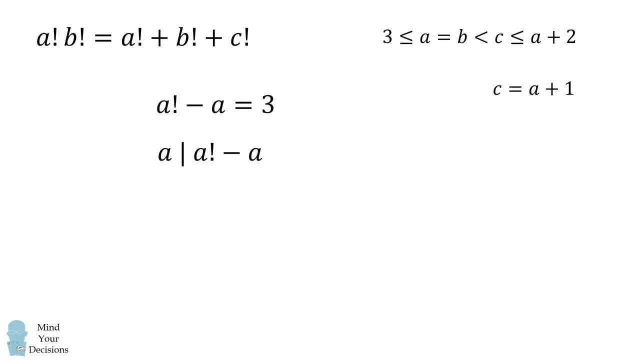 Now from this equation, a does divide a factorial minus a, which means that a would have to divide 3.. Since a is greater than or equal to 3,, this means that a is equal to 3.. So we now consider the positive equation. 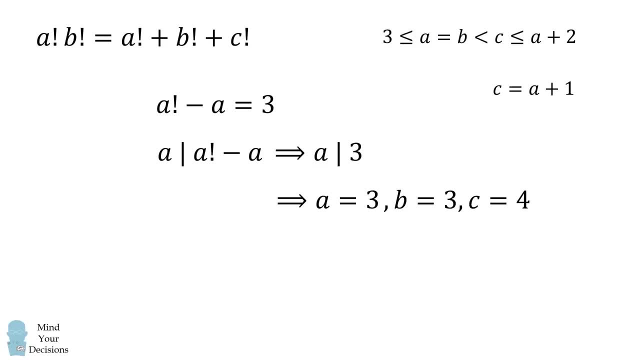 We now have the possibility that a is equal to 3, b is equal to 3, and c is equal to a plus 1, which equals 4.. We substitute that in to the original equation and, ta-da, We found the unique solution.